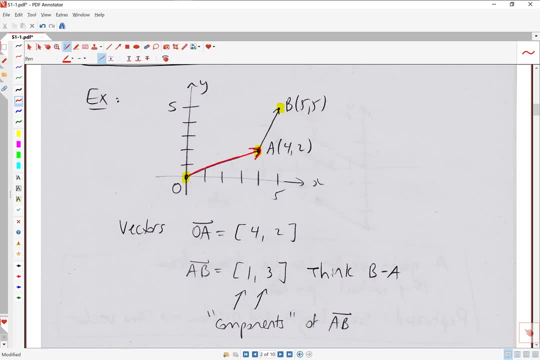 We've got a vector running from point O to point A and we've got a vector running from A to B. So let's talk about some notation that we'll use with vectors, and we'll also talk about how to calculate these vectors. 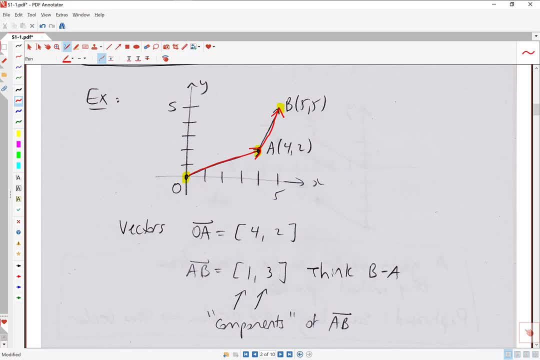 So when we write a vector running from A to B, for example, if we want to indicate that it's a vector, people will either write an arrow on top or sometimes it's easier just to write half arrow. So I tend to use the half arrow notation like that just to indicate that's a vector from A to B. 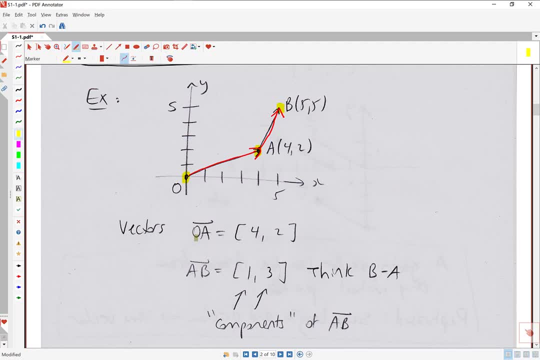 So if we look at the vector going from O to A, in notation we would just write it like this: And then let's think about: how far is it moving horizontally? Well, four units. How far is it moving vertically? Two units. 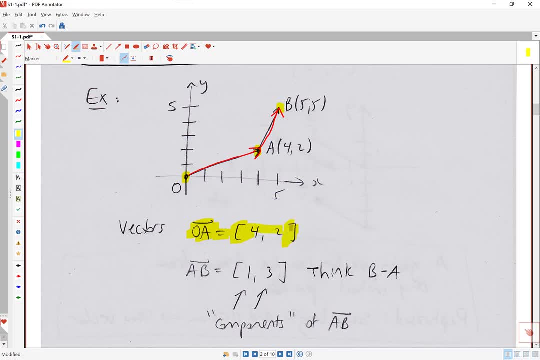 So the vector is written using square brackets and we just write the horizontal change and then the vertical change. So vector OA is this. This is the vector. The vector going from A to B is the vector, The way that we can actually calculate that. 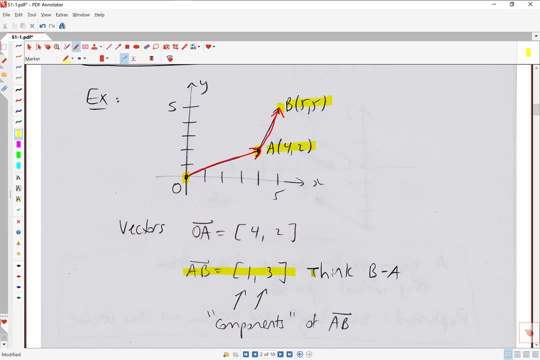 if we've got the coordinates of points A and B is just think B minus A. So to get the x component go, 5 minus 4 is 1.. So that's the net change in the x direction. And then 5 minus 2 is 3 to get the net change in the y direction. 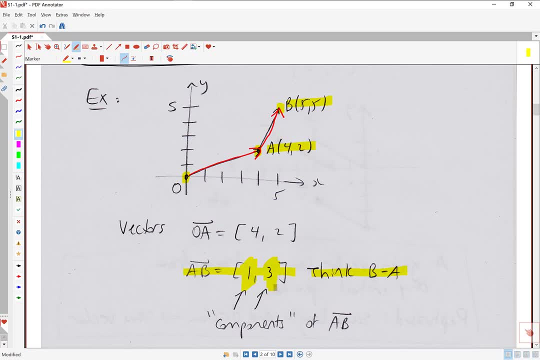 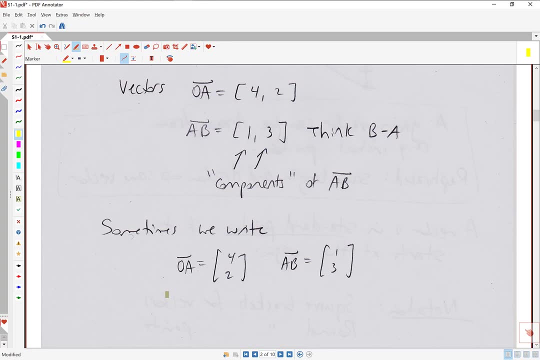 And these numbers that we're writing down inside the vector are called the components of the vector. So the components of vector AB are 1 and 3.. Now sometimes we write our vectors vertically, so you could equally well write OA as the vector. 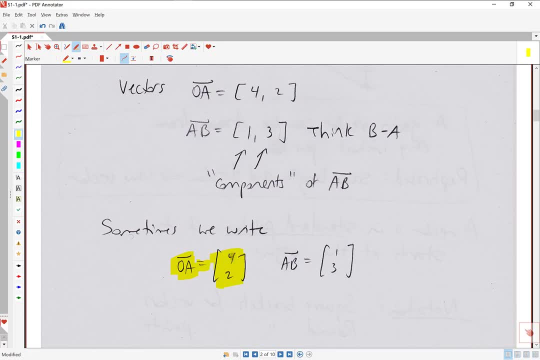 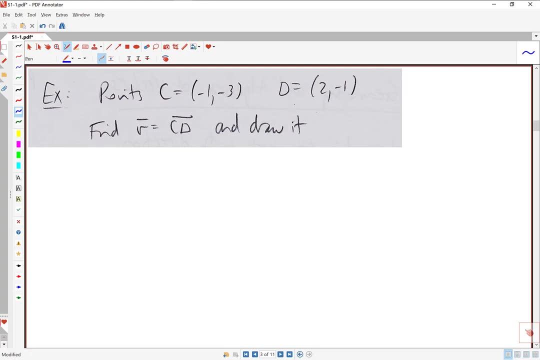 The horizontal component is still the one that's being written first. So this is going four units horizontally, two units vertically. So let's say that we're given points C and D and our goal is to find the vector from C to D. 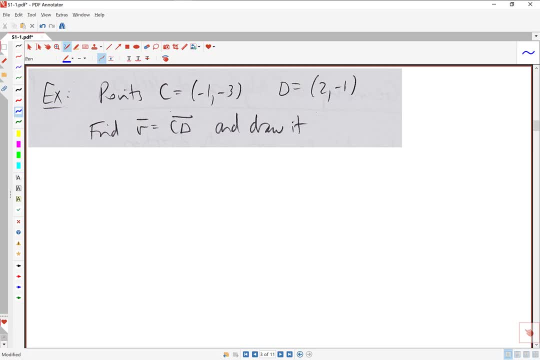 which we're calling vector. So we're going to calculate that and then we'll draw it. So let's say vector is equal to the vector that goes from C to D. The way we're going to calculate this, just think D minus C. 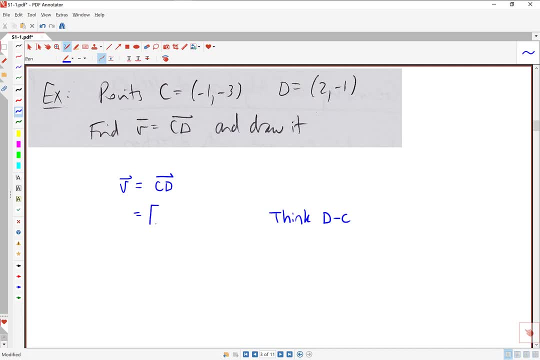 So we're going to go 2 minus. I'm going to write all the details here: 2 minus gives us our horizontal change and negative 1 minus gives us our vertical change. Okay, typically we don't actually write down that step. 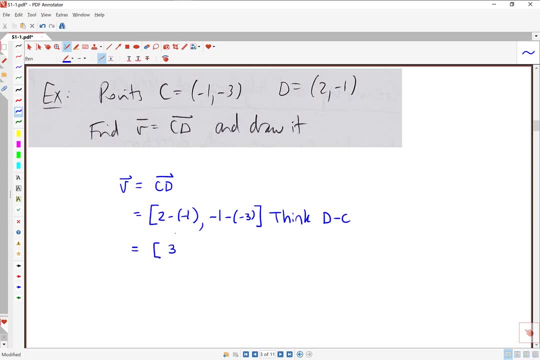 We just do that mentally. So the components of our vector B are going to be 3 and 2.. Okay, now let's think about how to draw that vector. So I'm going to draw the x and y axes here, So we could draw the vector starting at any initial position. 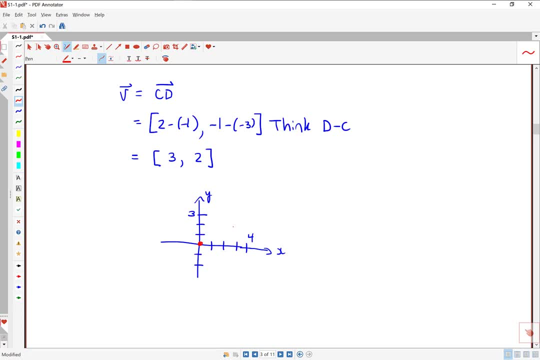 We could draw it starting at, and then it's going to move three units over two units up. So that's one copy. We could draw the vector, But similarly we could draw it starting at any starting position. So we could draw it starting down here. 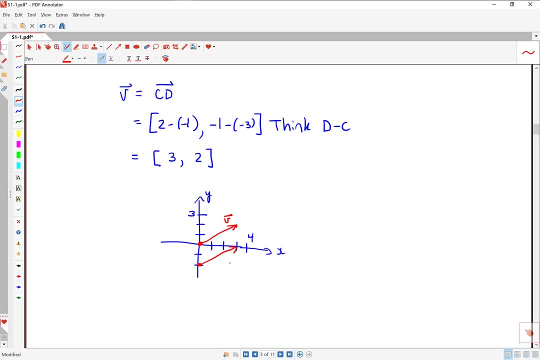 It's still going to go three units over two units up, So that's another copy of. We could draw it shifted over, starting here. It's still going to go three units over two units up, So that's So. there are infinitely many acceptable answers here. 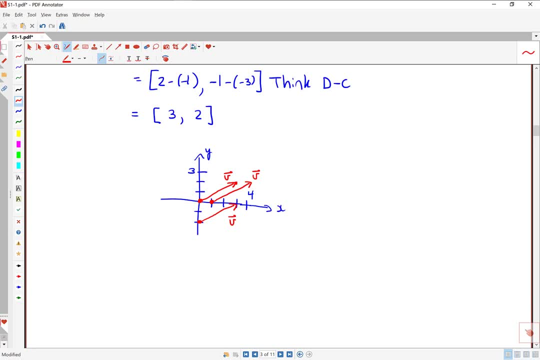 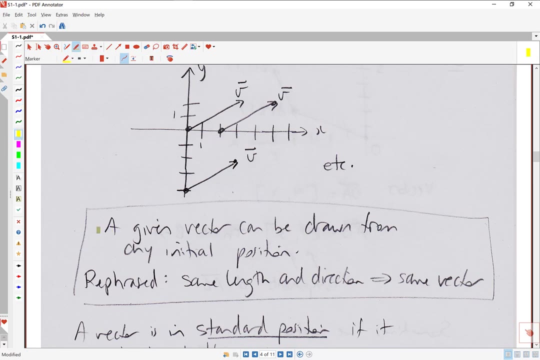 You can start this vector from any initial position and as long as it's traveling three units over two units up, then you've drawn a correct version of vector B. So let's make a couple of comments about this. What we figured out in doing that sketch is that a given vector 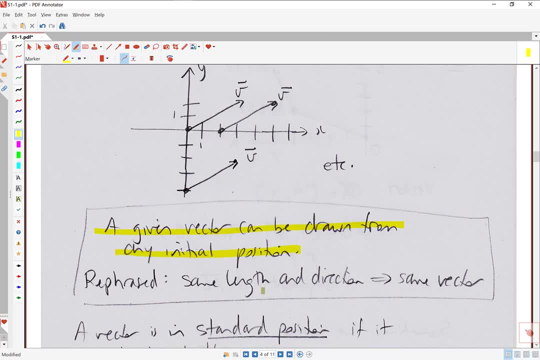 can be drawn from any initial position And if you rephrase that idea, that's like saying if two vectors have the same length and the same direction, that implies they should be called the same vector, They should be considered to be the same vector. 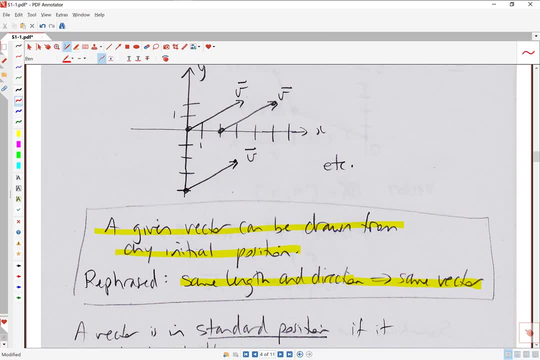 So in this drawing here we would not need to call these vectors- you know, V1,, V2, V3, because as soon as we call this one V1,, this one's V1, and that one's V1 as well, 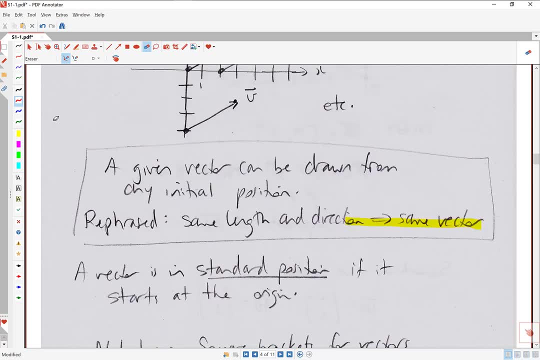 So we might as well just call them all V. Occasionally we want to draw our vector starting at the origin, just because it makes things easier from a geometric point of view. So a vector is considered to be in standard position if it starts at the origin. 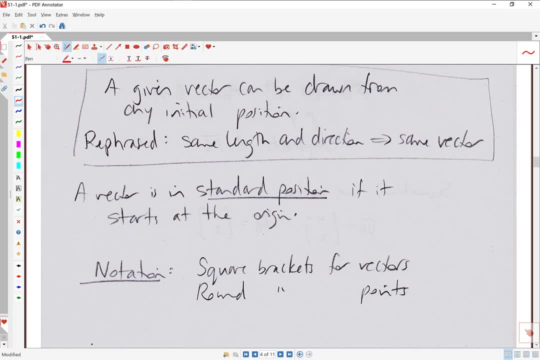 So at this point I want to talk about some notation that's pretty important going forward. So if someone writes down something like this, we should understand that that's a vector because it's got square brackets on it, whereas if we see something like this: 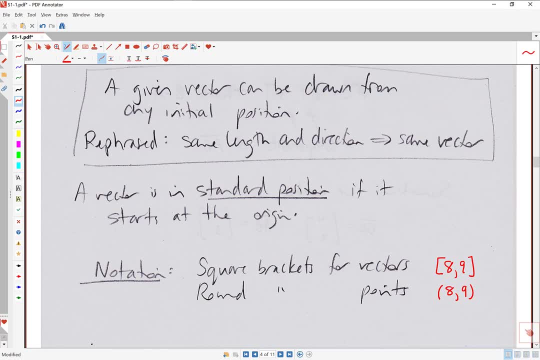 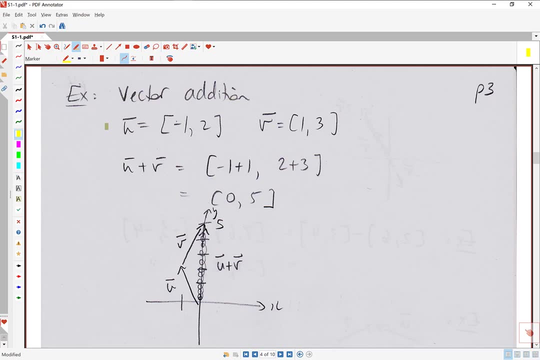 we should understand that. that's a point because it's got round brackets. So let's talk about how we add vectors to our model. Let's say we've got vector u and vector v given to us, So if we want to add these two vectors together, 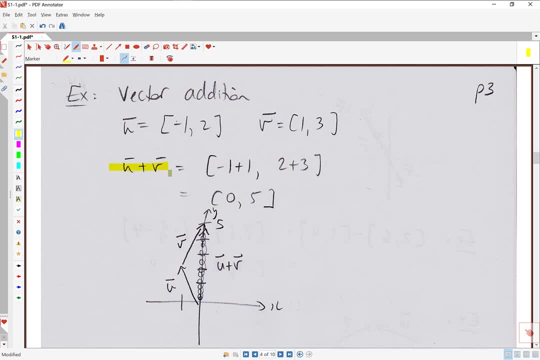 we'll call the sum vector u plus vector v, And what we're going to do is just add the x components together, so you'd get negative. 1 plus 1 gives you 0.. Add the y components together so you'd get 2 plus 3 gives you 5.. 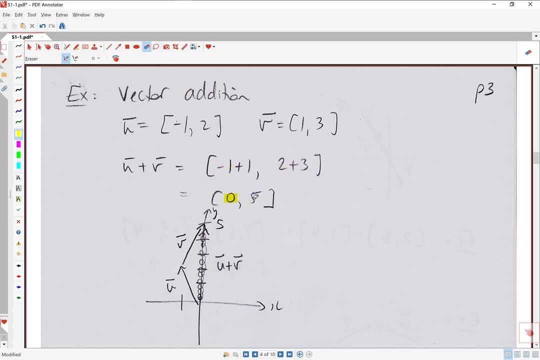 So that's the algebra of how the vector addition's going to work. But let's look at the geometry. So let's draw vector u. We can draw that in standard position. So it's starting at the origin. It's going one unit to the left and two units up. 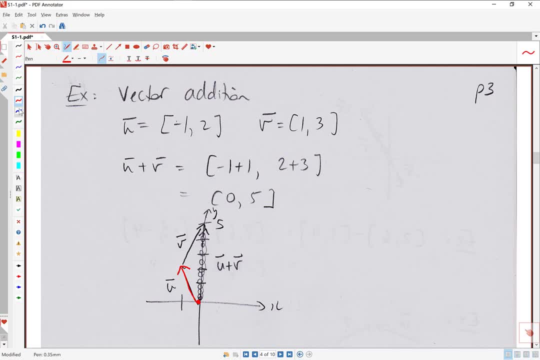 So there's our vector u And then, at the tip of vector u, we're going to start vector v. So starting vector v, here vector v is going one unit over and three units up. So that's what vector v looks like. 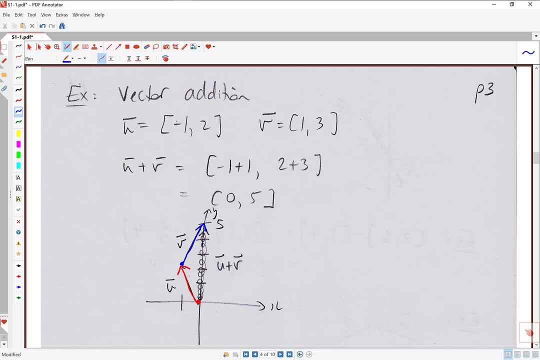 Okay, so this is called tip to tail. Whenever you're adding vectors, you draw the first vector and then at the tip of the first vector you're starting the tail of the second vector. So just position them like that And then to understand geometrically, 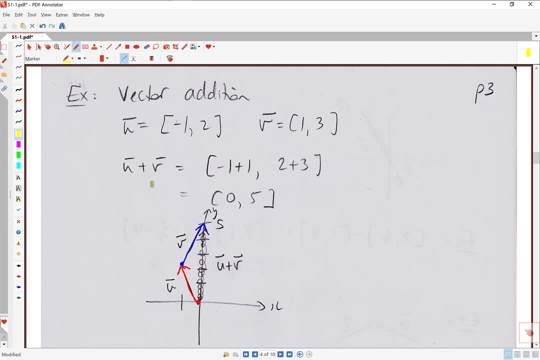 what the addition of the vectors looks like. the u plus v start where the first vector starts, so at the tail of the first vector and go all the way to the tip of the second vector and look at what vector we've produced. 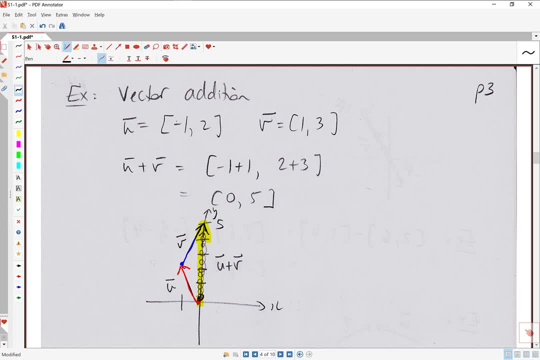 So we can see it highlighted here. I'm going to shade it in in darker markers so that we can see it. So it's going just five units vertically. That's our vector, u plus v, That's the 0, 5 that we created. 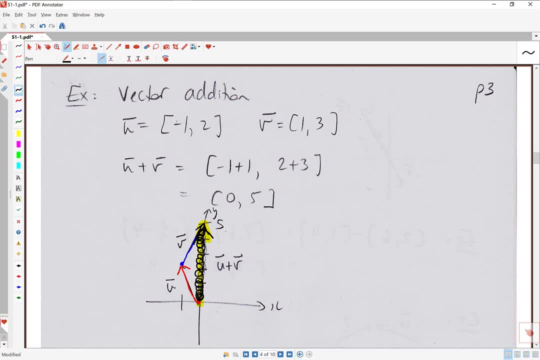 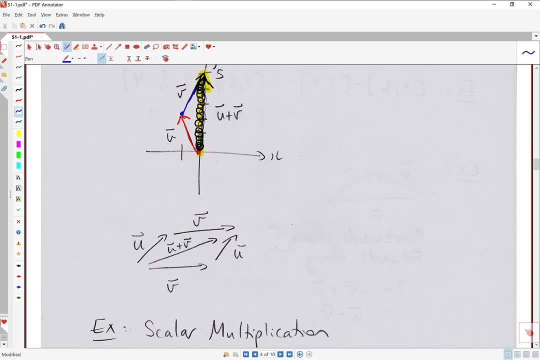 just by adding those two vectors together. So that's the geometry of how vector addition works. So maybe a cleaner way to understand that is just to draw a sketch without a coordinate system. One of the beauties of what we do in linear algebra is a lot of our discussion happens. 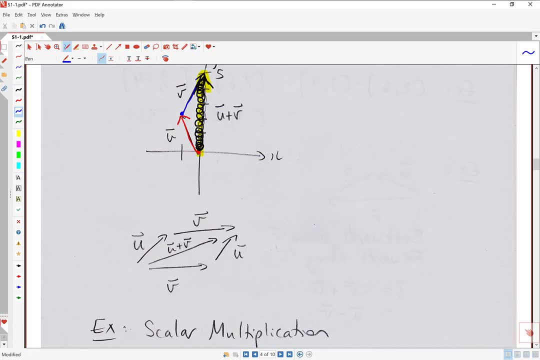 without even having any coordinate axes drawn, So we can just draw a vector like: oh, this is vector a, that's vector b, let's say So. to add these together means start where a starts, finish where b ends, and that's our vector: a plus b. 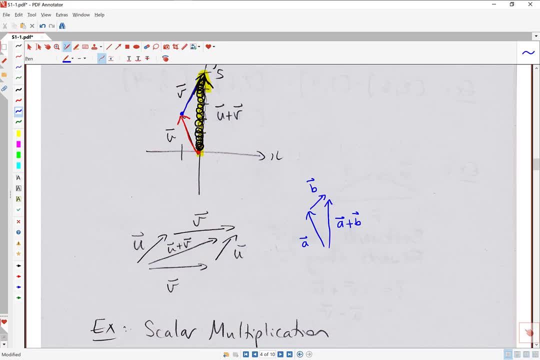 So that's the geometry of vector addition, And you can see that in this sketch that we've got here. So if you follow along u and then along v, what you're producing is u plus v. So one of the things that we can conclude from this picture: 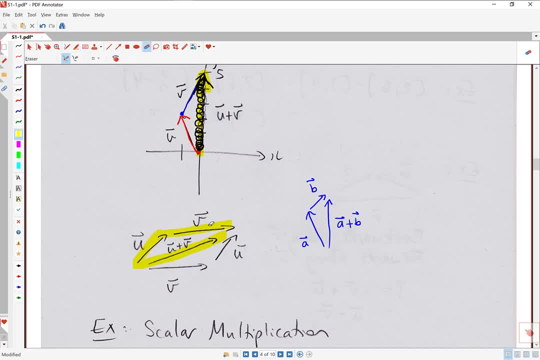 is that it wouldn't travel. it wouldn't matter if we travel along u and then v, or if we went in the other order. If we went along v and then along u, we would still produce the same vector, u plus v. So what we're concluding is that 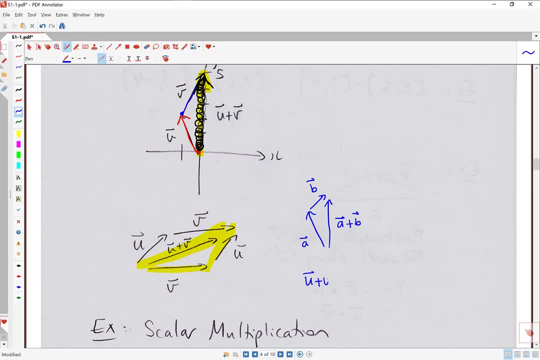 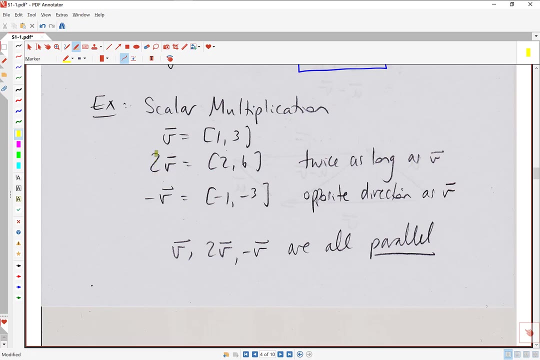 when we're adding vectors together, the order doesn't matter. u plus v is always going to be the same thing as v plus u, and we can see that from our sketch. Now let's talk about scalar multiplication. So scalar multiplication is when you do something like: 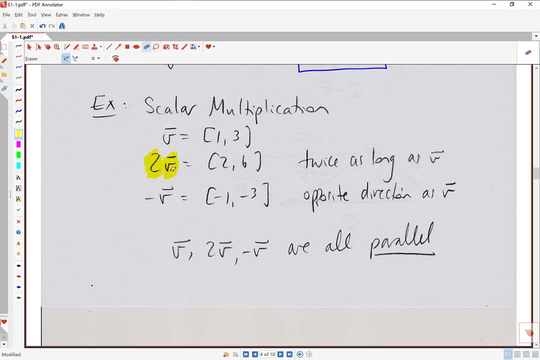 you multiply a number times a vector. Often a number is called a scalar, so that's where the name scalar multiplication comes from, just multiplying a constant times a vector. Okay, so let's say that we've got a vector v that looks like: 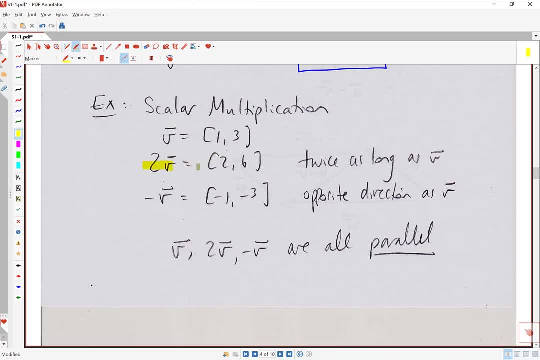 So to take two times that vector just means multiply each of your components by 2, so you would get. And while we have this algebra discussion, let's also have the geometry discussion at the same time, So we'll actually draw a picture here. 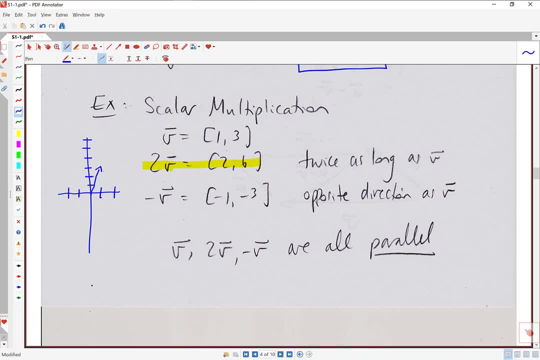 So let's say this is our vector v, and if we double that, what we're getting is a vector that's twice as long as v, but pointing in the same direction. So we're going up to. So red vector, here is 2v. 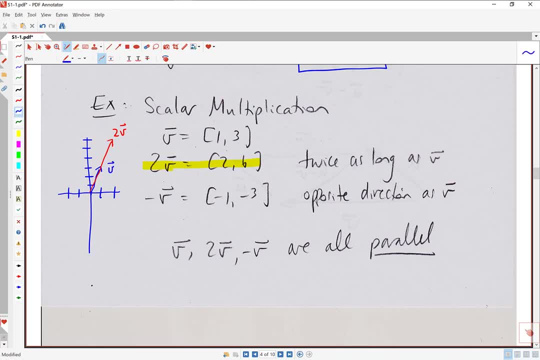 whereas the blue one was just v. So multiplying a vector by a positive scalar just makes the vector that much longer in the same direction, Whereas if we did something like algebraically, we're just changing the signs of the components and what that does is changes the direction of the vector. 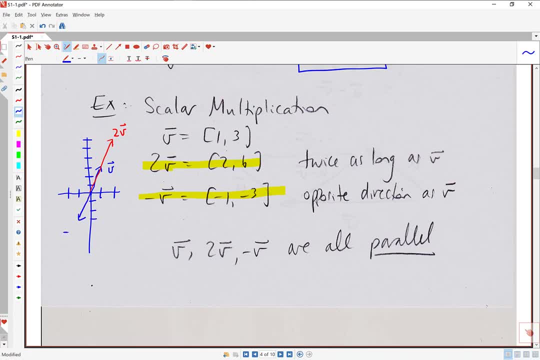 So we'd be going like this. So that's just as long as v pointing in exactly the opposite direction. So when we look at these three vectors- v, 2v and negative v- they're all considered to be parallel. 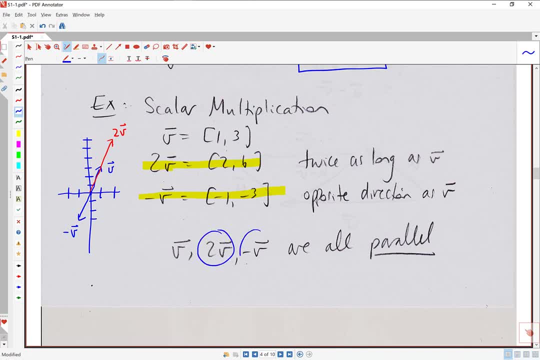 So even if two vectors are pointing in opposite directions, like 2v and negative v, they're still considered to be parallel because they lie along the same line. So vectors that lie along the same line are parallel. So we've talked about how to add vectors. 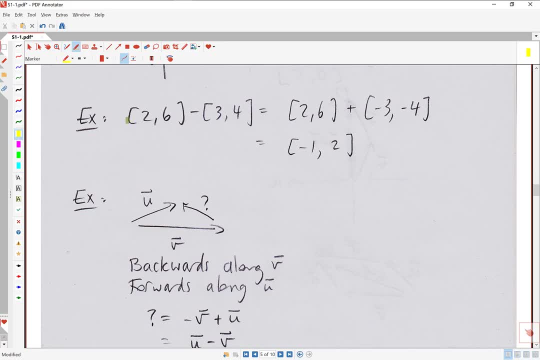 we've talked about how to scalar multiply and therefore we have all the tools we need to subtract One vector from another. So let's say we wanted to do Okay. so technically what we're doing here is we're multiplying the second vector by negative 1.. 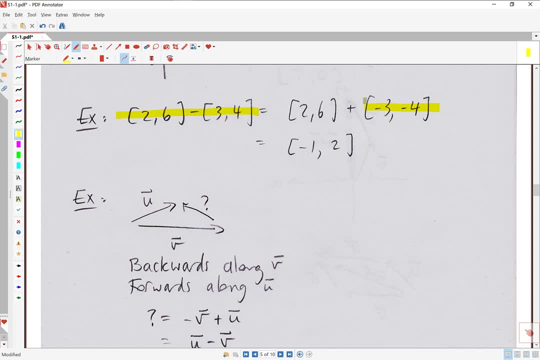 So that negative 1 just gets multiplied through and then it becomes a vector addition problem. So you would get Okay. now on a more intuitive level, I think most people would just say: okay, that just means do the subtraction on each component. 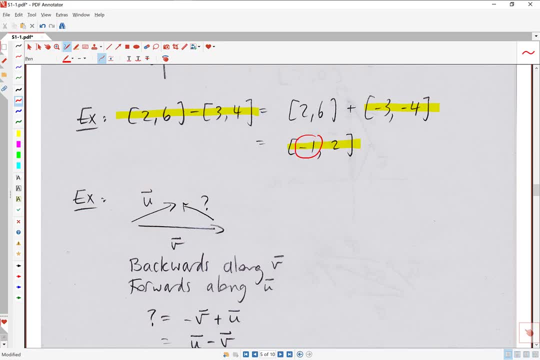 So you go 2 minus 3, gives you your negative 1, and you go 6 minus 4, gives you the positive 2.. And that's really the best way to think about vector subtraction. So let's look at the geometry of subtracting vectors. 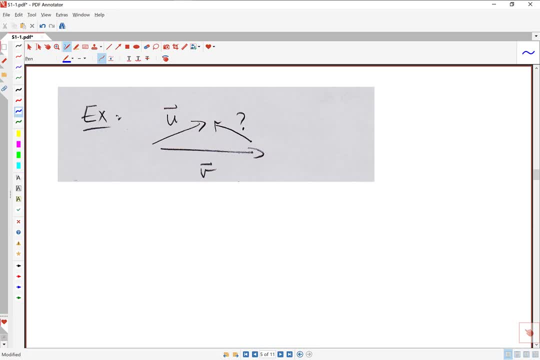 So we've got a diagram here showing vector u and vector v And we've got this unknown vector question mark that we want to describe in terms of u and v. So let's see if we can figure it out. So this question mark. 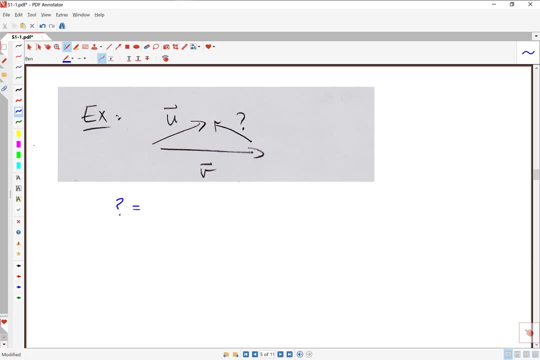 this unknown vector, let's describe what it does. So to say it goes this way is the same thing in vector language as saying: well, it must go backwards along v and then forwards along u. So let's see if we can express that algebraically. 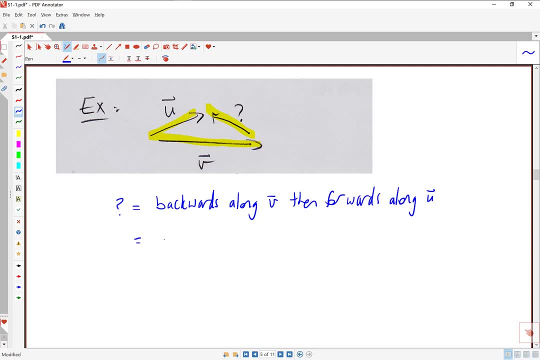 So when you go backwards along a vector, that's like saying you're traveling along negative v, because negative v is a vector that's just as long as v, but in exactly the opposite direction. So negative v, and then we would want to go forwards along u. 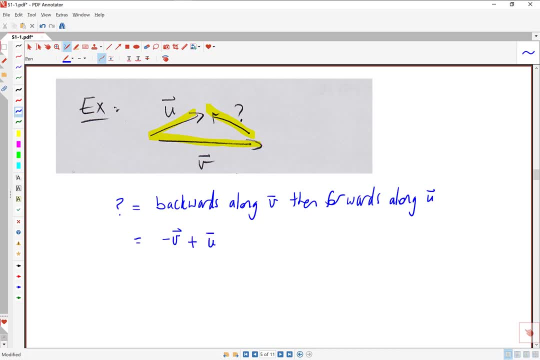 So when we say, then we're doing a vector addition and what we're adding on is vector u. So you could say negative v plus u, but I would say that's a bit more natural if you write it as u minus v, So we can encode this idea. 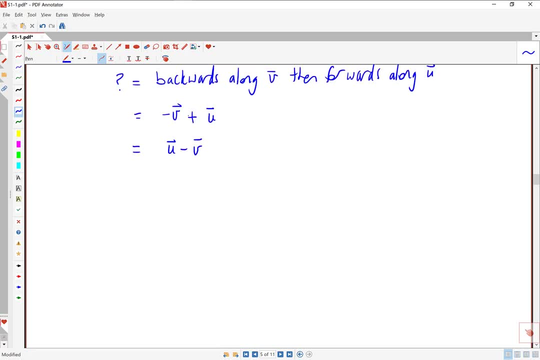 just with a different diagram here. Let's draw a bigger picture. So let's say: this is vector u, this is vector v. Often what we'll see is a parallelogram where we've got two copies of v, two copies of u. 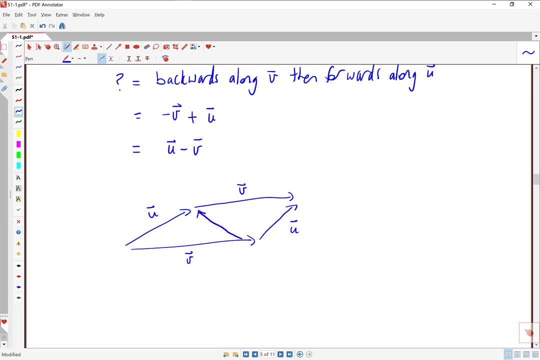 And what we've just talked about is the vector that goes this way. So that's the vector u minus v, And if you had decided to run that vector in the opposite way, so let's say instead, you wanted to talk about this vector here. 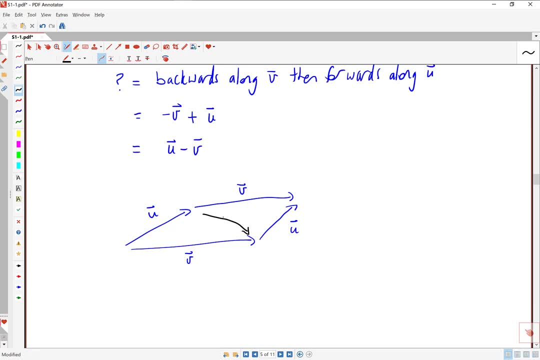 Well, one way to think about it is: well, it would just be the opposite sign of what we just talked about, So it'd be negative u plus v, which we might call v minus u. But the way you would actually figure that out geometrically, 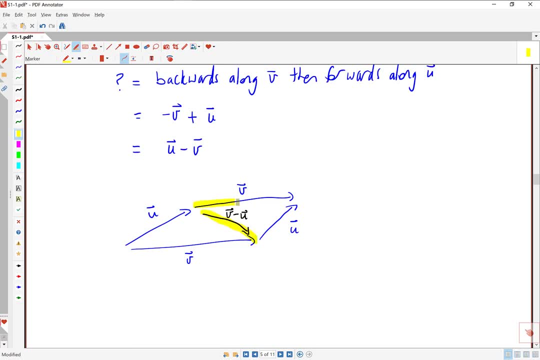 is. you'd say: well, what would I need to do to create this vector? I would need to travel along v and then go backwards along u, So v minus u would be the best way to say that. So notice that we've talked about the addition. 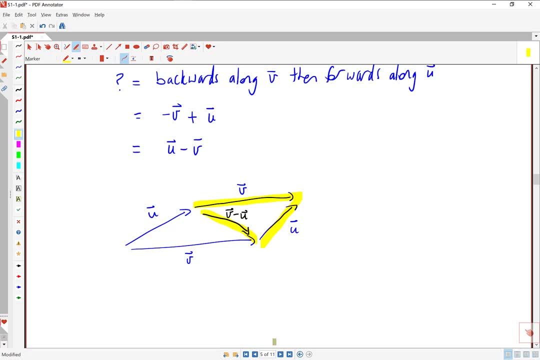 subtraction, scalar multiplication of vectors, And for each of those topics we've looked at, okay, how does the algebra work, How does the geometry work, And this is going to be a theme throughout the course, Pretty much every topic that we look at. 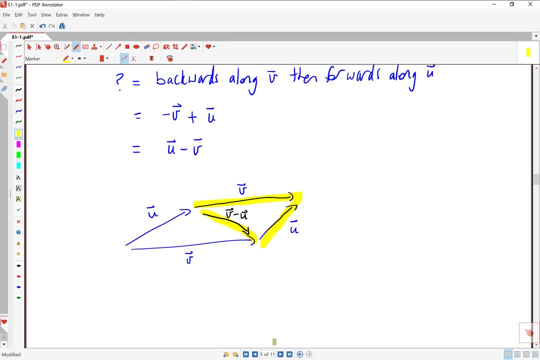 we're going to look at the two sides- the algebra and the geometry- and just try to weave them together. So here's one more problem involving vector addition. Often we'll have three vectors in the mix, And what we'd like to do here is draw u plus v plus w. 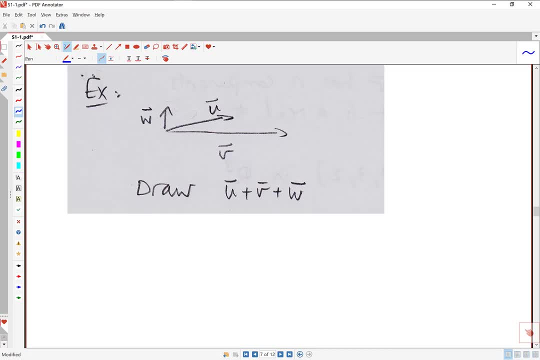 So the way I would approach this is: I would just think about drawing u plus v first. So let's imagine that vectors u and v define a parallelogram, because it's just so nice that the sum will be a diagonal of that parallelogram. 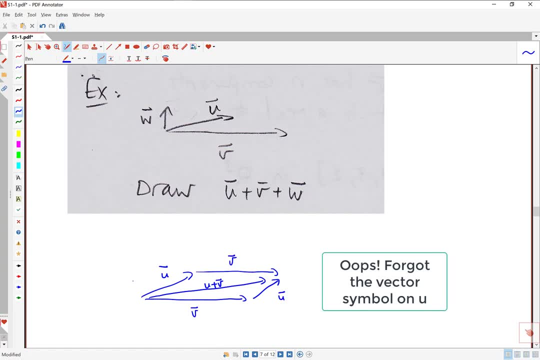 So that's our u plus v there, And w is a vector that goes just straight vertically like that. Now remember that a given vector can be positioned at any starting point. So in our diagram we saw w sitting over here, but there's no reason that it needs to be over there. 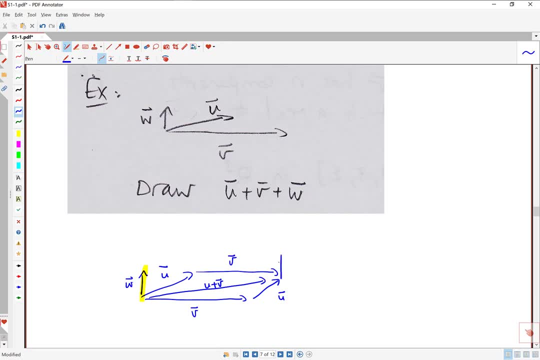 If we would now like to add w to u plus v, then we really want to imagine w sitting over here. So we're just going to reposition w, still going the same. it's still got the same length and same direction as it did originally. 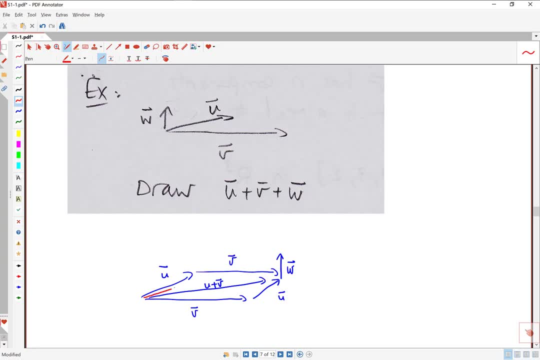 And now we can add w to u plus v. So we're going to get this vector here that starts where u started and that finishes where w ends, And so this big red vector here, that's u plus v plus w, So geometrically, if you wanted to imagine. 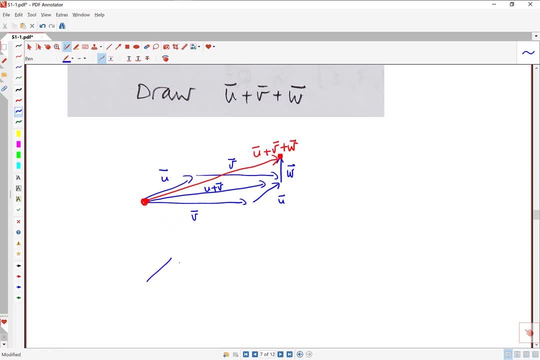 that u, v and w form a box. I'm going to draw it for a second without the arrows, just so that it's a little bit cleaner. So think of u and v as forming the base of the box, and then w is here helping to create the sides. 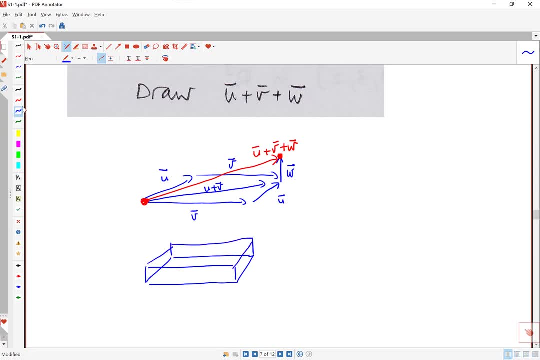 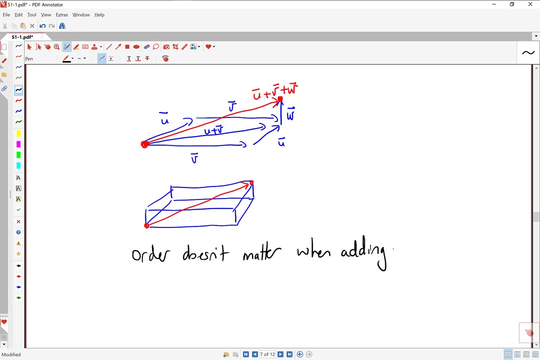 So we've got this box that looks like this: Then u plus v plus w is just starting at one corner and going all the way to the opposite corner. And again, what we can emphasize in this diagram is that order doesn't matter when adding vectors. 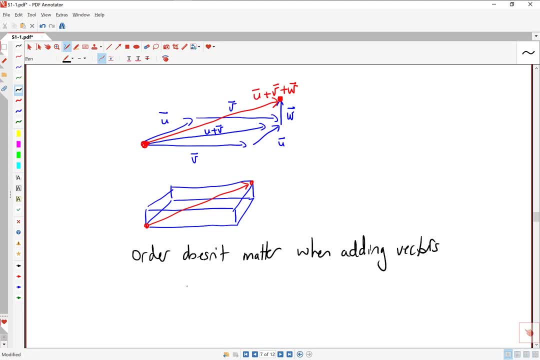 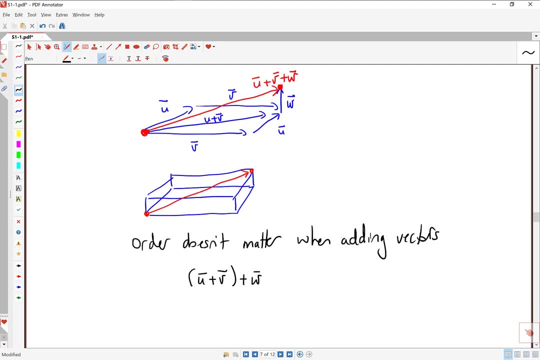 because technically what we did was we chose to do u plus v first and then we chose to add w to that. But you can check that if you decided on another order you would still create the same vector, For example. let's say we wanted to try. 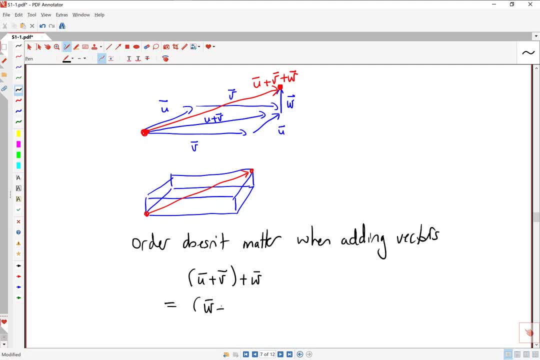 w plus u and then add v to that later. So let's do a little bit of labeling in this sketch here. So w is the vector that goes up vertically, u is the vector that goes back and v is the vector that goes over. 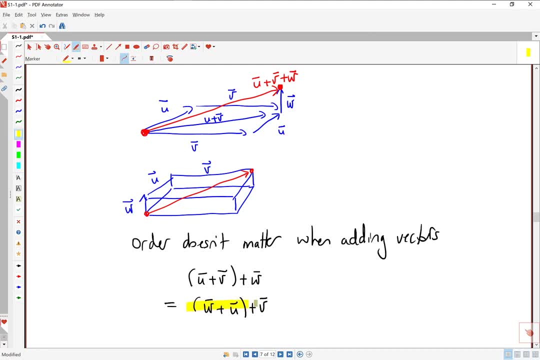 Okay, so if we decided to do this order here: w plus u and then plus v, we would go: w plus u creates this vector that goes diagonally along that side there, And then if we added v to that, we would still be creating this big red vector. 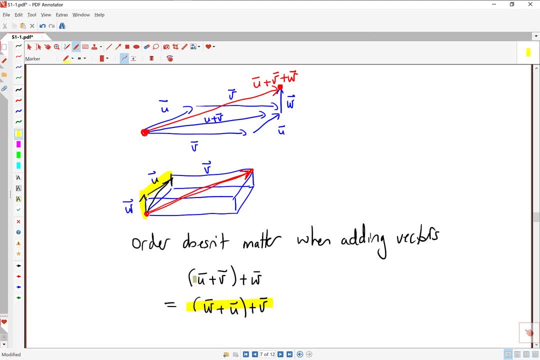 which we said is u plus v plus w. So I'm just going to write et cetera here, Because if you try doing this in any one of the six possible orders, you will always be creating that same red vector. So as long as we're adding vectors, 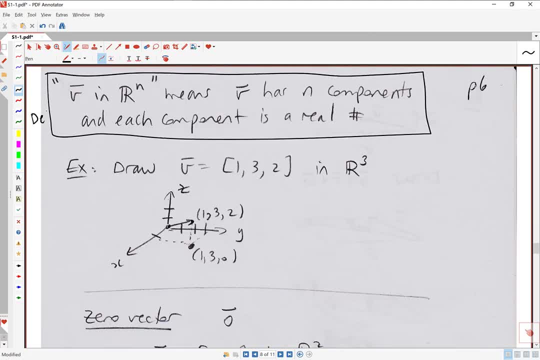 order does not matter. Now let's look at a quick definition. This is a piece of notation that we'll see a lot in linear algebra. When we say something like v, vector v is in Rn, what that means is that vector v has n components. 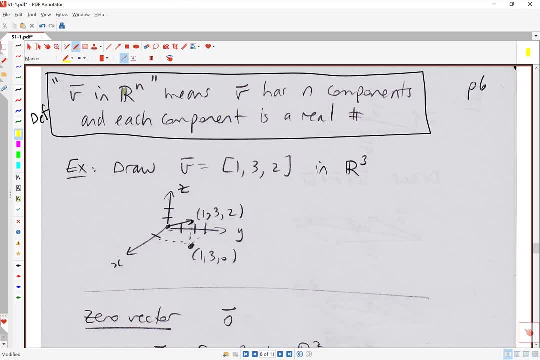 and each component is a real number. That's what the R represents, But, to be honest, it's really the number of components that's important to us. So the two situations that we'll see a lot is where we have a vector in R2,. 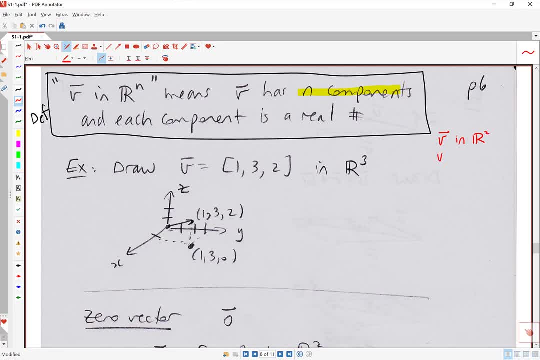 so we're just drawing the x-axis, the x-y plane. We'll also see situations quite frequently where v is in R3, which means we're drawing three-dimensional space. So it just gives us a clue as to what dimension we're working in. 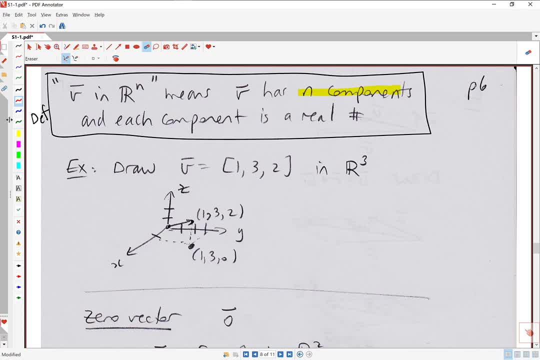 So let's do a little bit of practice here with drawing vectors in three-dimensional space. We'll just do a quick example. So let's say vector v looks like and we're going to try to draw this in three-dimensional space. So I think I'll redraw the diagram. 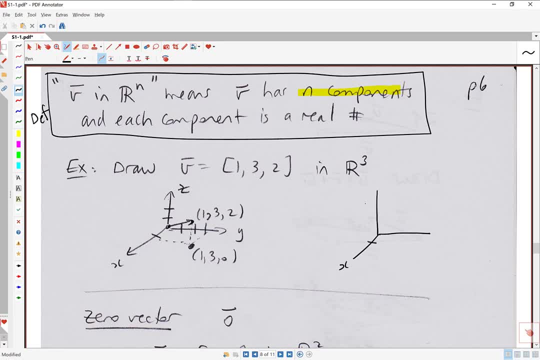 and put it aside so that you can see this developing. First thing we should probably talk about is our axes. So the typical way to draw the x-y-z axes for our course is to imagine that the x-axis is just coming straight out of the page at you. 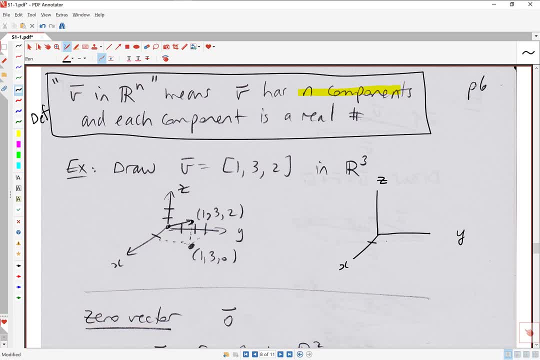 So we usually draw it slanted like this. So x is coming right at you, y is going to the right and z is going up. There are different courses. different textbooks will use different orientations for the axes, but we'll stick with this orientation here. 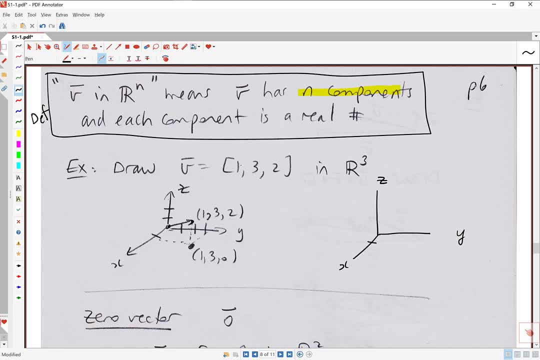 So, with that discussion done, let's see if we can draw a vector that's just going one unit in the x direction and three units in the y direction. I won't actually draw the vector yet, I'll just draw the point. Let's find the point. 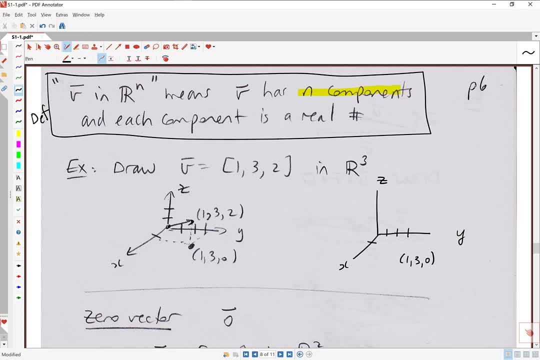 So to show this in 3D, what you can do is imagine the x and y axes, sort of forming a parallelogram like that. You could say: that's the point, And then if we want to create the point from that, then we need to measure what looks like two units. 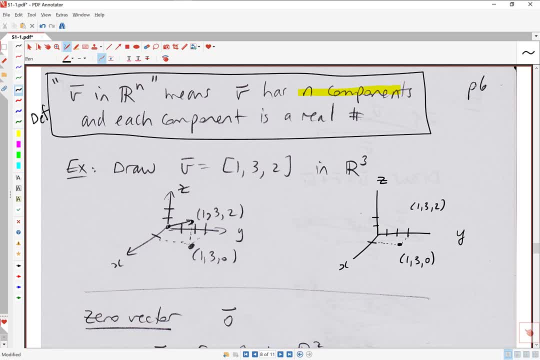 along the vertical axis. So just sort of eyeball that distance, So looking at this and sort of just measuring that distance there And then travel that distance from the point vertically. So I would say it would be about there, That would be our point. 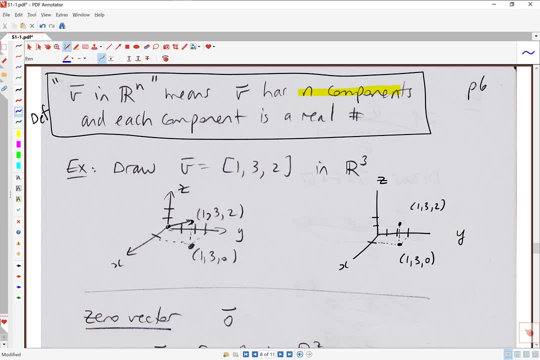 And once you can draw points in 3D, then of course you can draw a vector in 3D. So this vector is just starting at the origin and going over to that point. That's what looks like, So we can call that vector. 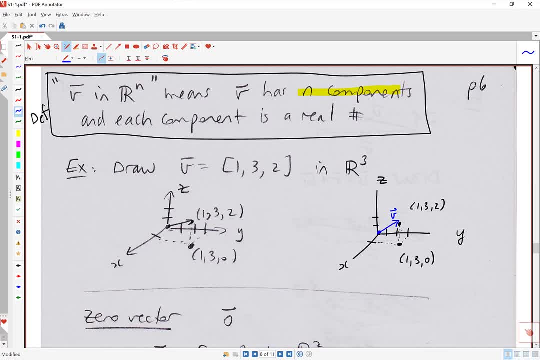 Most of the time, we'll be doing our diagrams without a coordinate system, but it is helpful to be able to do a clear sketch in 3D when you need it. Okay, let's introduce another definition here. We're going to talk about the zero vector. 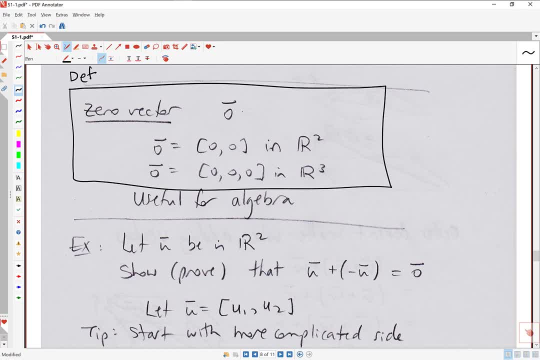 which we're going to write the number zero, with the vector sign over it. If you were in R2, then the zero vector would look like. If you were in R3, then the zero vector would look like. So, from a geometry point of view, 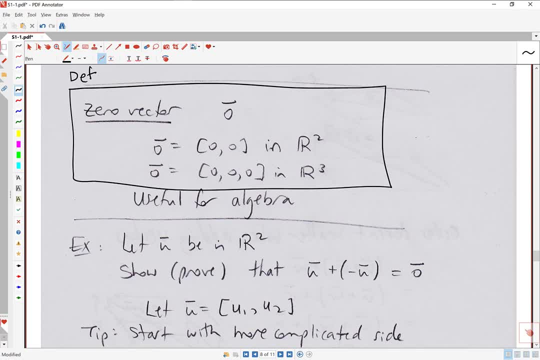 the zero vector is not very interesting because it starts somewhere and just finishes at that exact same point, So it's not a very interesting vector to work with, But it is actually quite useful for algebra, especially when we're coming up with formulas. So we'll see that throughout the course. 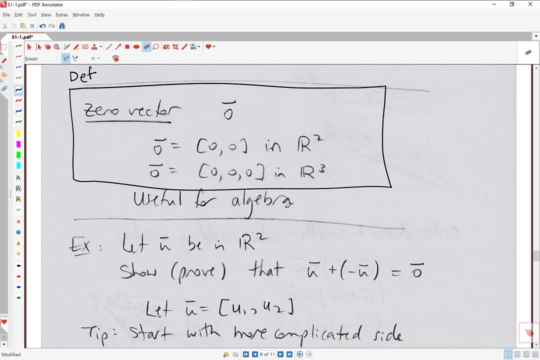 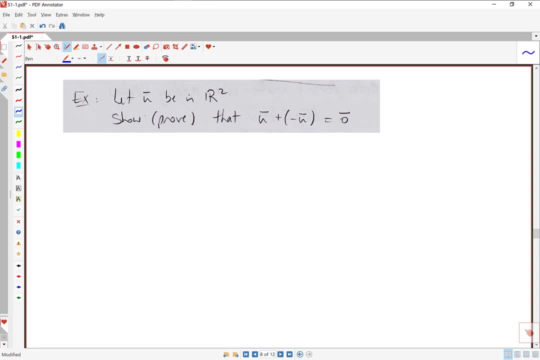 that the zero vector is going to be quite important. Let's do just a quick example to reinforce what the zero vector is. So here's our example. We're told: let vector U be in R2.. We want to show that U plus negative U. 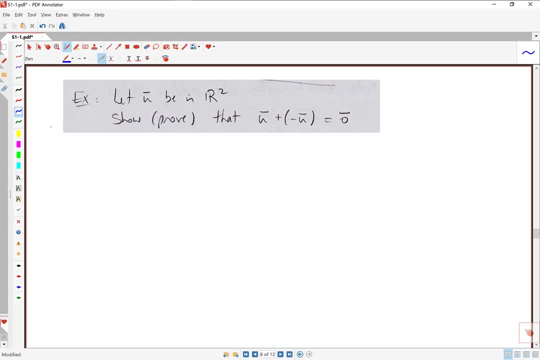 gives us the zero vector. So in this context you could say show, you could say prove. It's kind of scary, They mean the same thing. So essentially we just want to confirm that this equation is true Occasionally throughout the course. 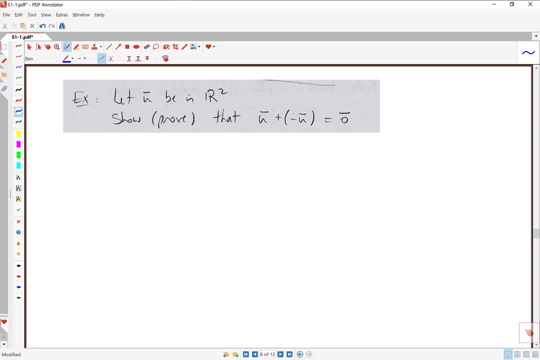 there will be a few instances where we have to do this sort of thing, where we're checking that an equation is true. So let's figure out how we would go about this. First thing we should do is we should just make U a bit more specific. 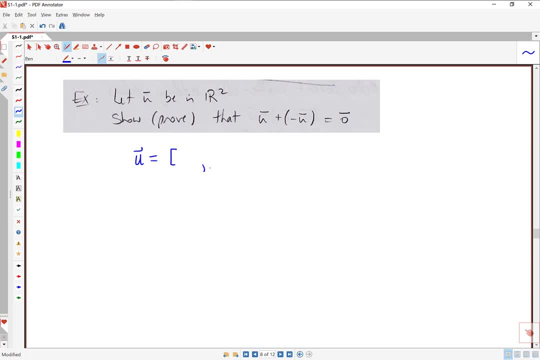 We're told that U is in R2, so we know it has two components. So it'd be nice to give a name to these two components so that we can actually do some algebra. And the usual way to do that is if your vector is called U. 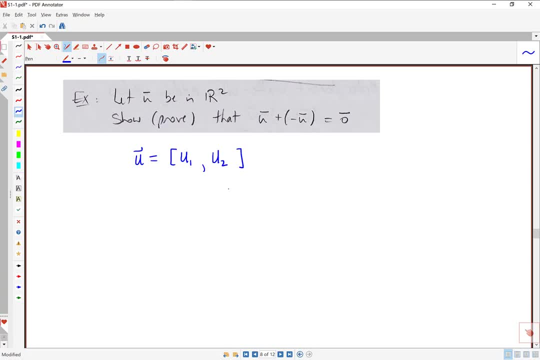 usually we call the first component U1 and the second component U2.. So we can say, let U be that. Okay, now we've got some numbers to actually calculate with, And when you want to confirm that an equation is true, generally, what you want to do is start. 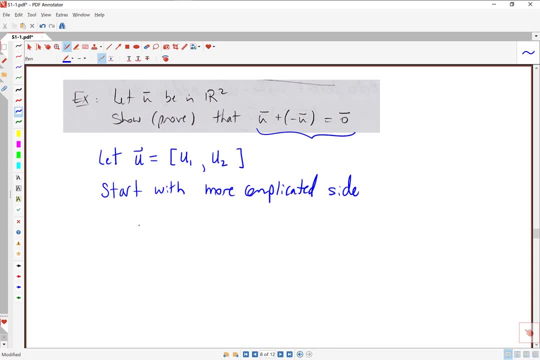 with the more complicated side. So I would say that would be the left side. I would start with vector U plus negative vector U, And what we're trying to do logically is, through a sequence of steps, we're trying to create the right side. 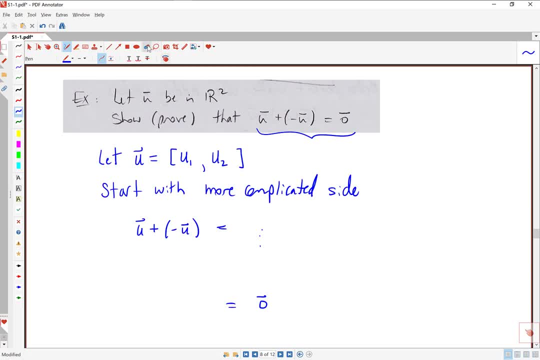 So if we can do that, then we've shown that these two things are equal. Alright. so first step, we're just going to use the fact of what U is, U is U1 comma U2.. So we're going to add U to negative U. 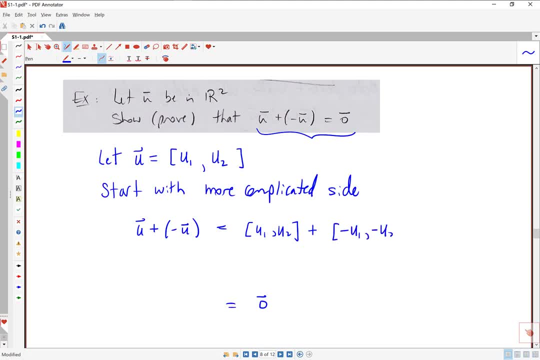 Okay, well, negative U is what you get if you just multiply the components of U by a negative, And then we're going to do our usual addition: U1 minus U1 would be 0.. U2 minus U2 would be 0.. 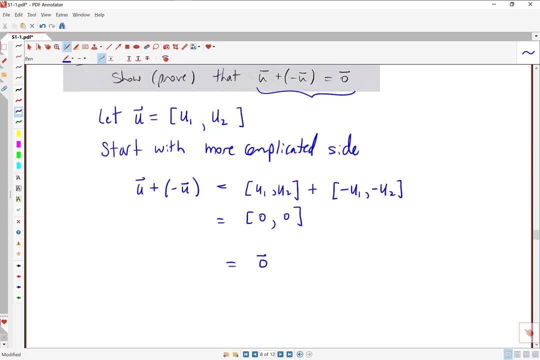 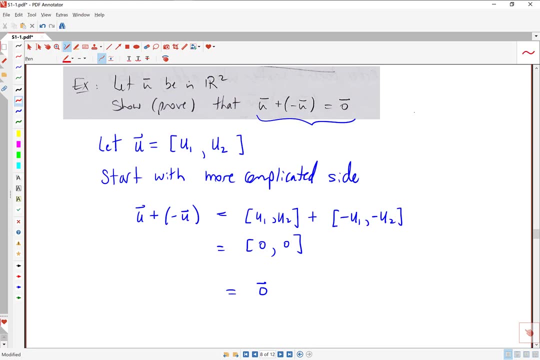 So, sure enough, that gives you the 0 vector. So I would say, geometrically, the idea that we just showed was obvious, So geometrically obvious that if you start with any vector U and then you run backwards along that vector, that you're just going to get back to where you started. 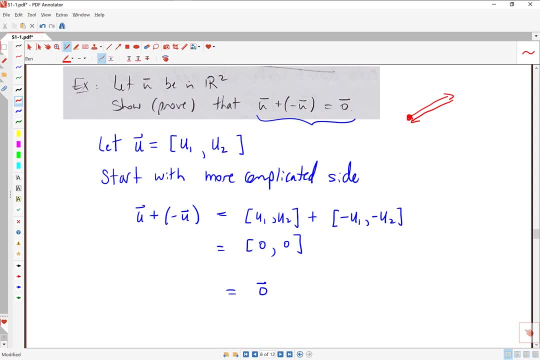 In other words, you're creating a 0 vector, But there are places in linear algebra where we do want to confirm a formula just from an algebra point of view, Even if something is geometrically obvious. So that's what we're emphasizing here. 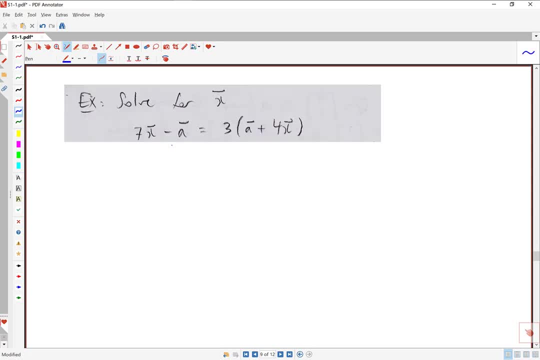 Alright. next example: Let's solve for vector x in the following vector equation: The main thing we need to know here is that we're going to follow the usual arithmetic rules. So, for example, you can attribute the 3 on the right side to say 7x minus a. 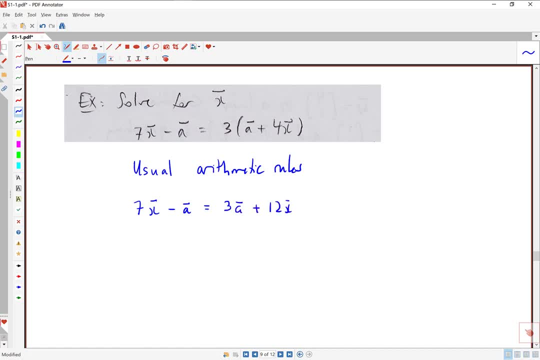 equals 3a plus 12x. You can add a to both sides, so you can say 7x equals 4a plus 12x. At the same time you can subtract 12x from both sides, So negative 5x equals 4a. 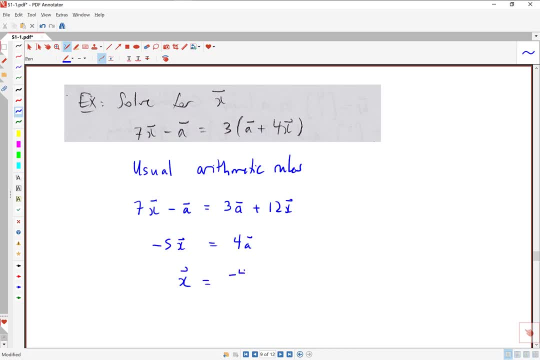 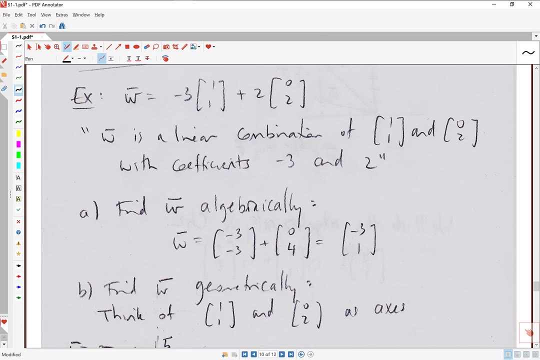 and then you can divide both sides by negative 5.. So x equals negative 4 fifths of a. So just a quick example to illustrate that you're distributing a constant or adding, subtracting, dividing. all work as usual. Next example: Let's say: 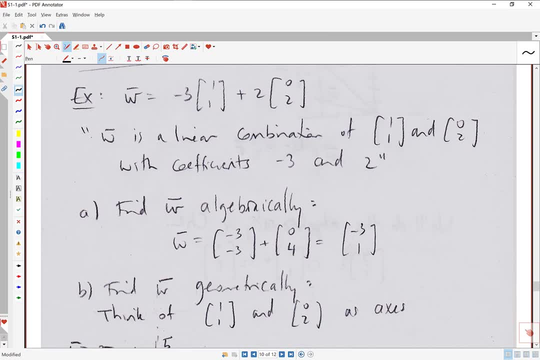 w is written as a sum of two vectors, And this is actually a really common setup in linear algebra, So common that I want to define a definition, a piece of terminology, just to talk about this setup. So the setup we're looking at is where we've got. 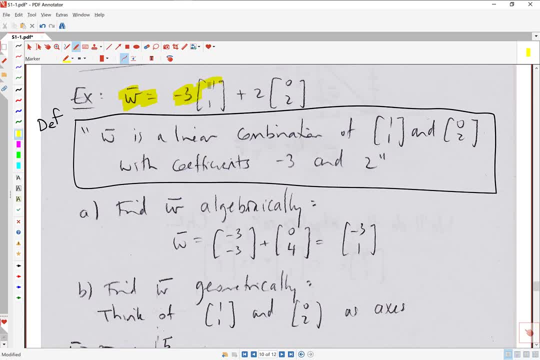 a vector equal to some constant times a vector plus another constant times another vector, So really common setup. When you see that setup we're going to say, w is a linear combination of 1, 1 and 0, 2 with coefficients negative 3. 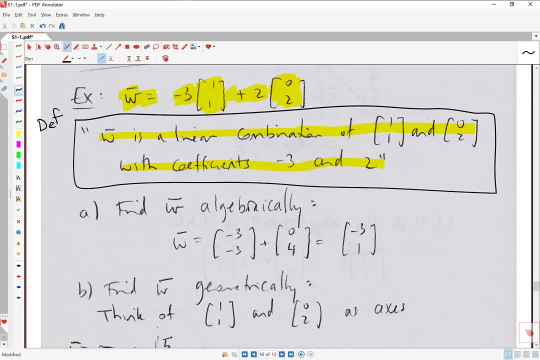 and 2.. So the main piece of terminology to pull out of this is linear combination. So you've got a linear combination when you've got some vector. let's say v is equal to a number times a vector. let's call it. 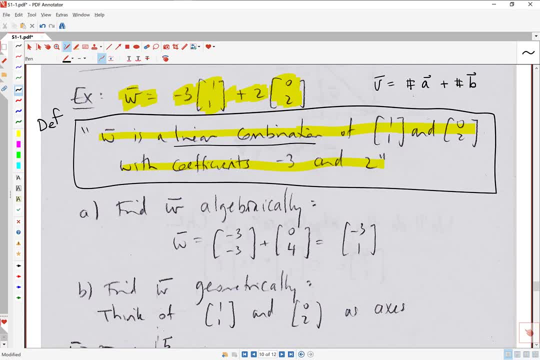 a plus another number times another vector. We would say vector v is a linear combination of vector a and vector b. So with this setup we're just going to do a couple of quick calculations. What we're going to do in part a, find w algebraically: 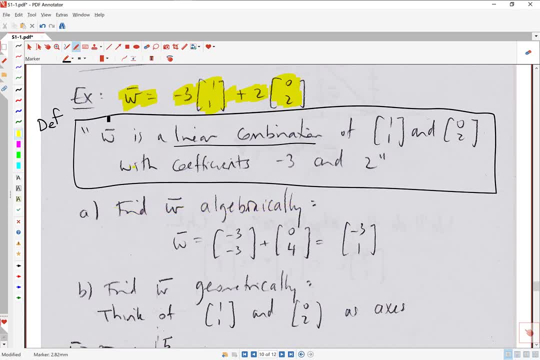 Okay, so that just means take the highlighted stuff that we can see in the question. let's just do a little bit of simplification on the right side and figure out what w looks like. So we would multiply the negative 3 through. we would multiply the 2. 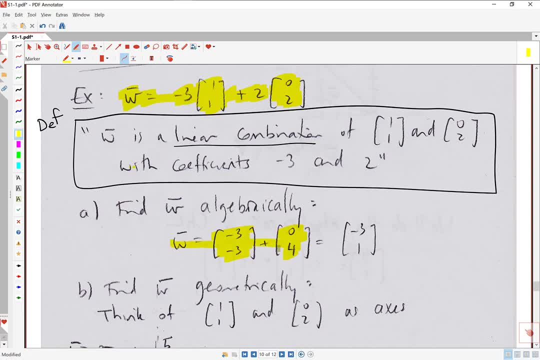 through the second vector. so we would say w is equal to that sum, which works out to negative 3, 1.. So that's from an algebra point of view how we would find w. But we could equally well find w geometrically And 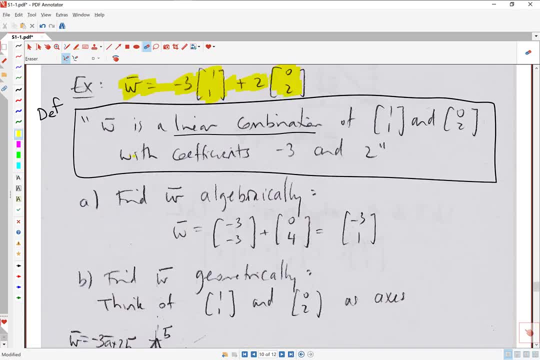 this, I think, is where things get a little bit more interesting. So what I'm going to do is just copy on the side here what we were given so that we can scroll down the page. So w was negative 3 times 1, 1. 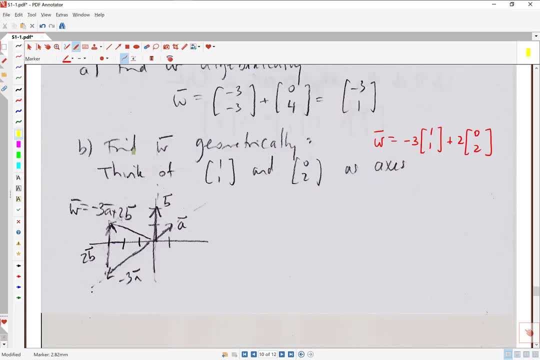 plus 2 times 0, 2.. And we're going to try to find w geometrically Okay. well, the idea is to think of these two vectors, the 1, 1 and the 0, 2, as giving us new 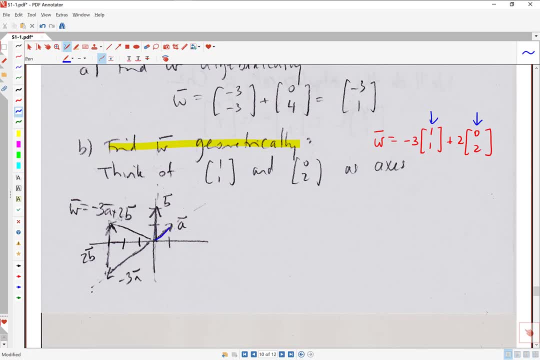 axes for the problem. So we've essentially got a 1, 1 axis here and we've got a 0, 2 axis here. If you want, you can call these a and b, Because if you do that then you can just label them more quickly. 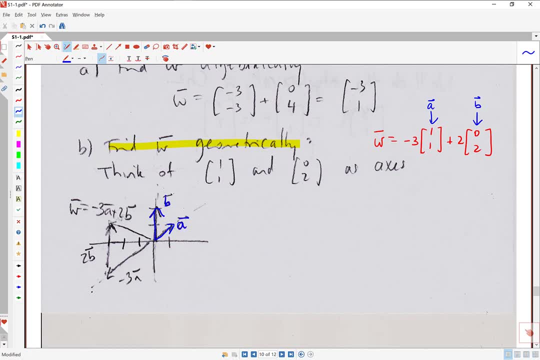 in the sketch. So we've got this a vector and we've got this b vector, Okay, and what are we trying to do? We're trying to figure out what happens if we go negative 3 times a. Okay, so that's the opposite. 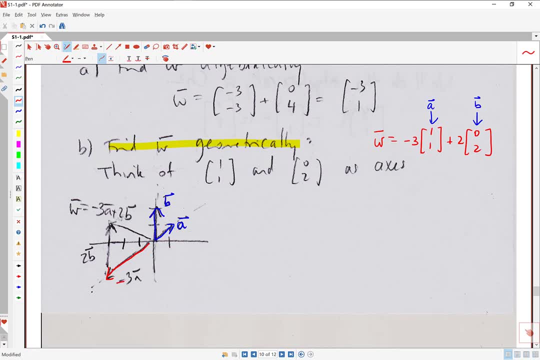 direction of a 3 times as long. So there's our negative 3a, And then we're going to go plus 2b, But we're going to be adding that to the vector negative 3a that we just built. So starting at the tip, 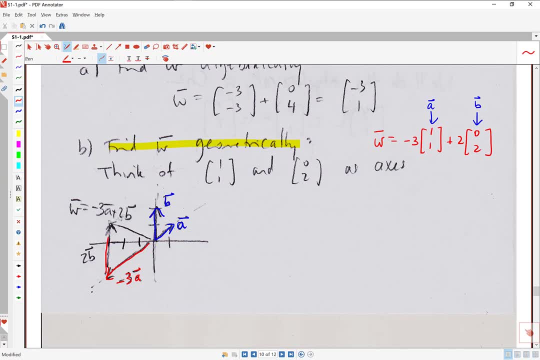 of negative 3a, we're going to go 2b, So that's going to be twice as long as b, but in the same direction. So there's our 2b, And to add these together just means position these tip to tail and look at. 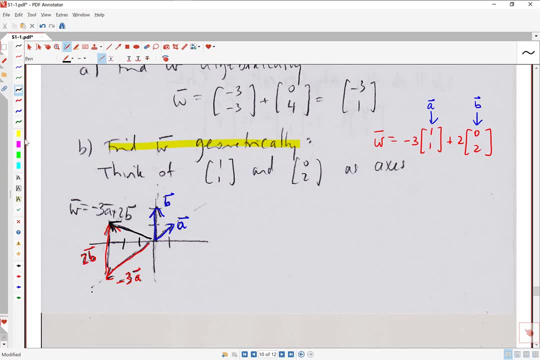 the result. So the result is this black vector. here I might highlight it, You can see it more easily. That is our vector w, Negative 3a plus 2b. So notice how the actual x and y axes became irrelevant here. 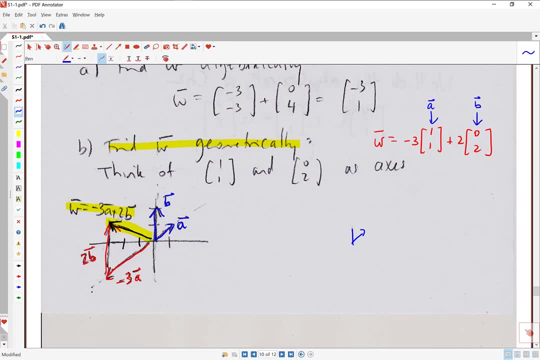 We didn't need them. So we had vector a going like this, We had vector b going like this And we said, negative, 3a looks like that, 2b looks roughly like that, And so, therefore, we can build our vector w. 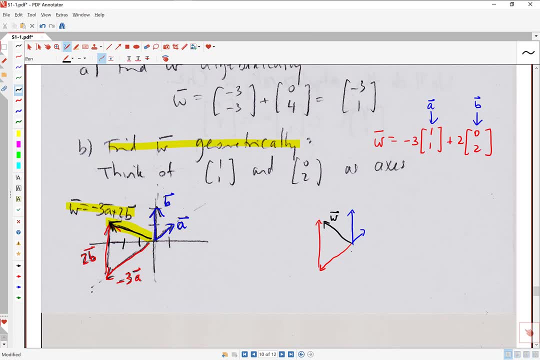 like that. No x, y coordinate system needed, Just vector a and vector b. So to find a linear combination geometrically means: forget about your original axes and just think about your new axes that are formed by your two vectors, And then go correct distance along each of those two. 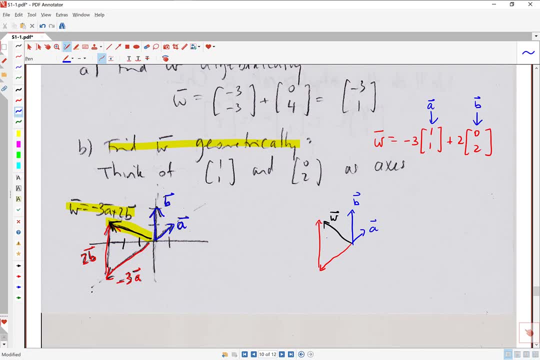 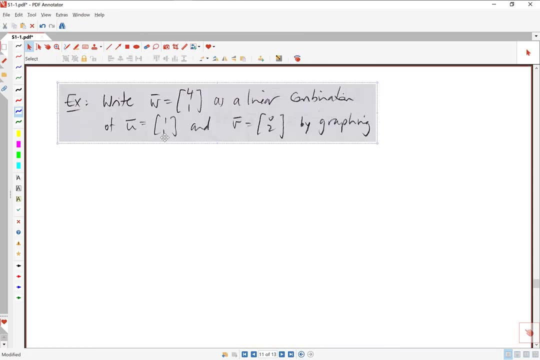 vectors to build your vector w. So let's put this into practice with a bigger example. So let's write the vector 4,1 as a linear combination of the vector 1,1 and 0,2 by graphing. So the fact that it says: 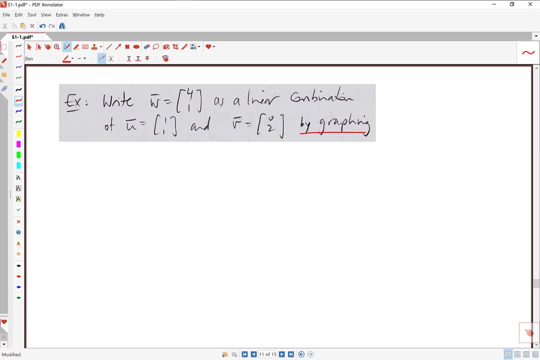 by graphing means treat it as a geometry problem rather than an algebra problem. So what's going to be important here is the vector u, which is 1,1.. So let's label that, And the vector b, which is 0,2.. 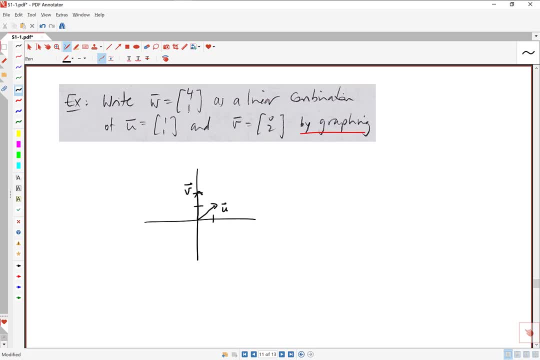 So we'll label that, And then we could also draw the vector that we're trying to build, which is vector w, which is 4,1.. So let's draw that one in red, just for contrast here. So that's the vector w that we're trying to build. 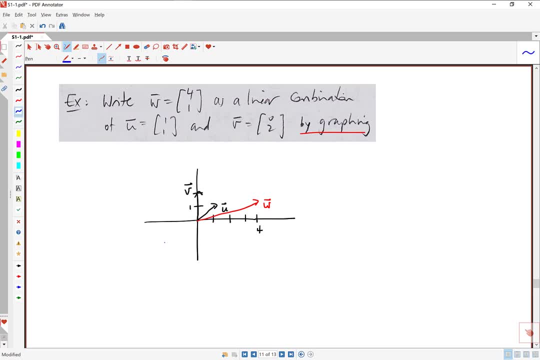 So what we're allowed to do is we're allowed to travel any distance we like along u, either forwards or backwards, And we're also allowed to travel any distance we like along v, either forwards or backwards, And we're allowed to do sums of these things, So you can, for example, travel: 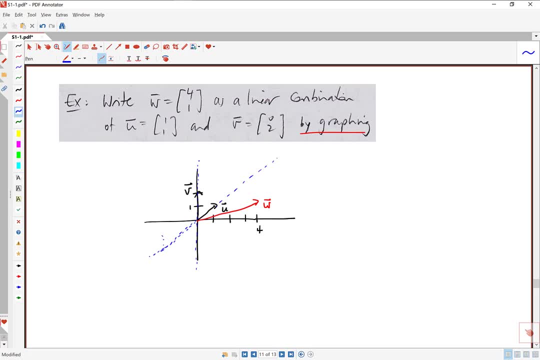 along u. You can say: okay, I'm going to go backwards along u and then I'm going to go either forwards along v or backwards along v, for example. So let's start at the origin and let's try to figure out a path that's going to take us to the 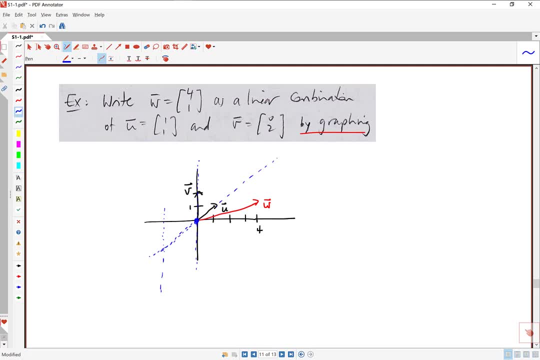 tip of w, So we could travel along u a certain distance, exactly the right distance, so that we're then going to be able to travel along v, So probably to about there, And then v is running straight up. We would like to run straight down. That's fine, That'll be equivalent. 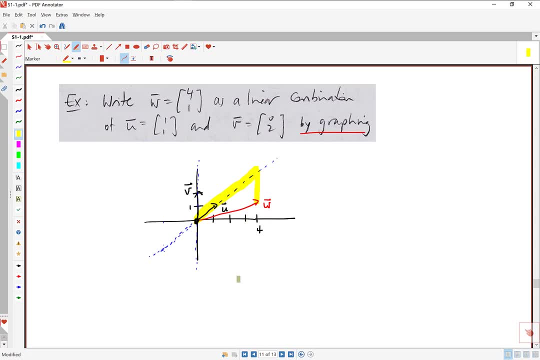 to going backwards along v. So that's sort of the path that we want to take. And then let's just eyeball this. So if we had drawn a careful enough sketch, we should be able to figure out the exact multiples to go along these vectors. 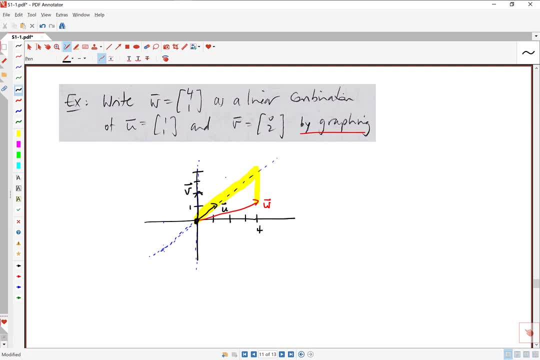 So it looks like we traveled from the origin up to the point four four. So I would say we went four times u. So at this point we're at four four and we want to come down to four one. So we need to travel three units. 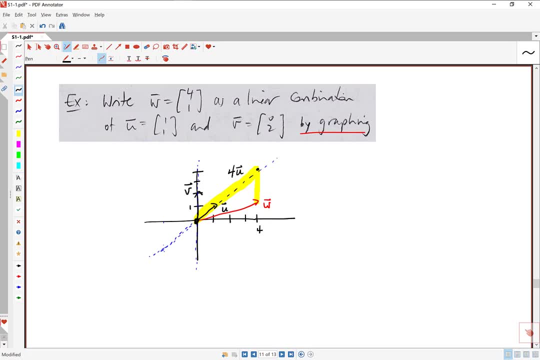 down and we need to do that along v. So if you're good with your mental math you would say: okay, that's going to be negative three halves of v. If you want a little bit more detail, then over on the side you could say, okay, I want to figure out a. 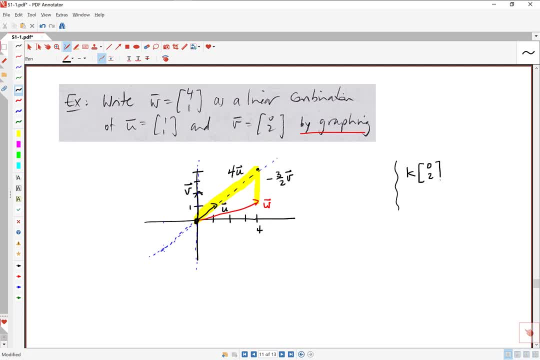 multiple of v. So I want k times zero two to equal zero negative three, Because what we're trying to create is this downward motion of three units And then we could say: well, if we just look at the second component here, that's like saying we want k times two. 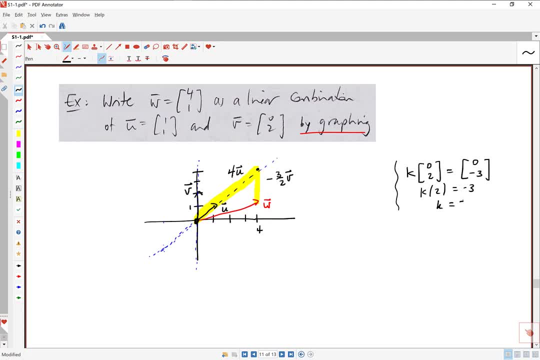 to equal negative three. So this multiple k should be negative three halves. So that's how we know that this should be exactly negative three halves. Alright, and so to answer the question, to write w as a linear combination of u and v, that means write w as some number. 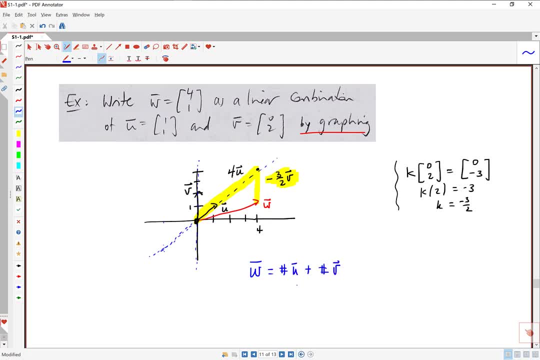 times u plus some number times v. That's what a linear combination of u and v is, And we've actually figured out the correct numbers. so we need to go exactly four times u, and then we need to go exactly minus three halves times v. And there we go. we've. 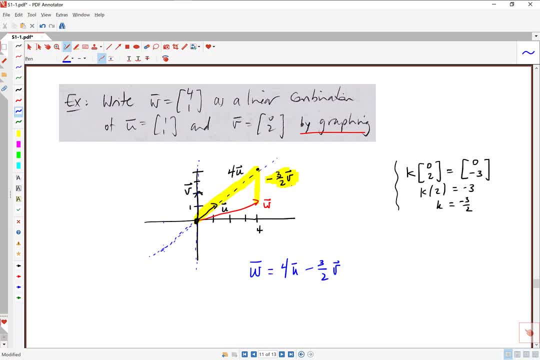 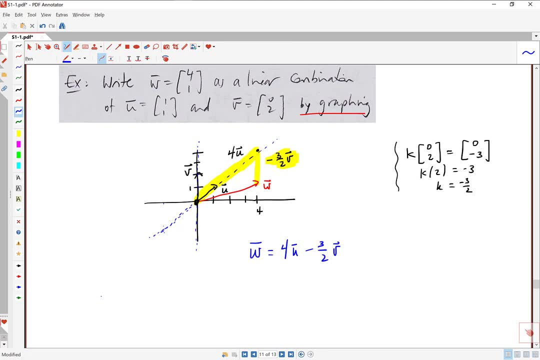 written w as a linear combination of u and v, just by drawing a picture. So you might wonder: hmm, how can we do this from an algebra point of view? So later on in the course, in chapter two, we'll have the tools to do this, If you wanted. 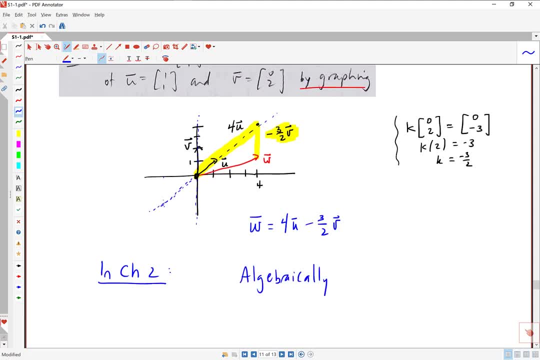 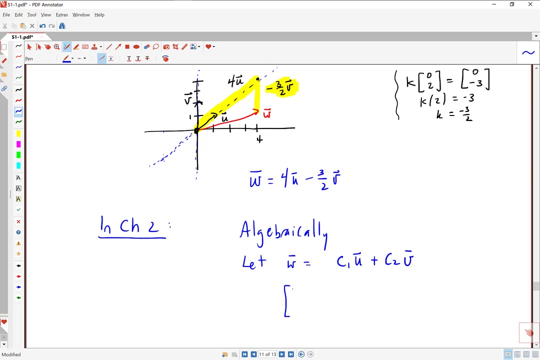 to do this algebraically you would say: let w be some unknown number times u plus some unknown number times v. We would usually call those unknown numbers c1 and c2, and so that would create a vector equation like four one equals c1 times one, one plus 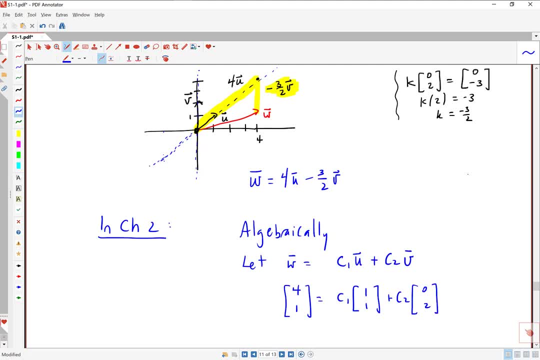 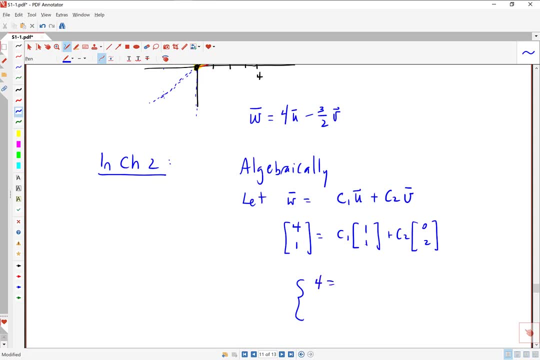 c2 times zero two. and what that's going to do is actually give us a system of equations, because you get one equation for the first component that says four has to equal c1 plus zero c2, and then you get a second equation from the second component that says: 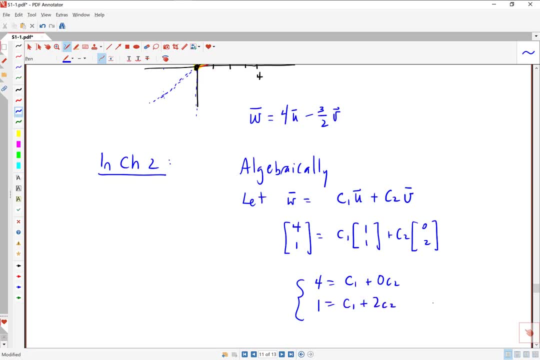 one has to equal c1 plus two c2, and then we'll talk. chapter two is all about solving systems of equations. so from there you could solve that system and get your coefficients. But if we did that algebraically here we would be missing the point. 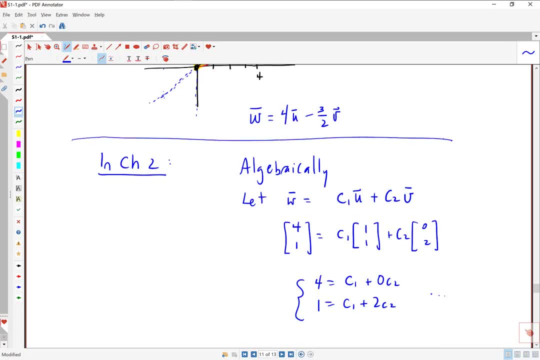 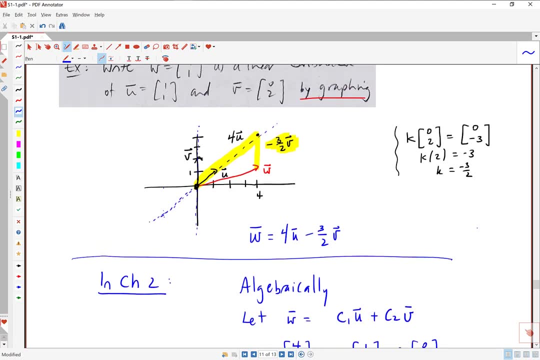 because the point of what we're doing in this section is just the geometry of the linear combination, so let's focus on just doing it using the picture. So we're going to do one last example here, just to make sure that we're brushed up on our trig. 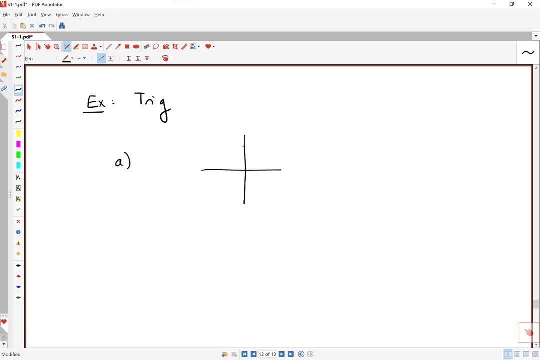 So part a: let's say we're given a circle centered at the origin that has radius five, and let's say that we've got a vector that's making a thirty degree angle with the positive x-axis. let's call that vector u, and what we want to do is: 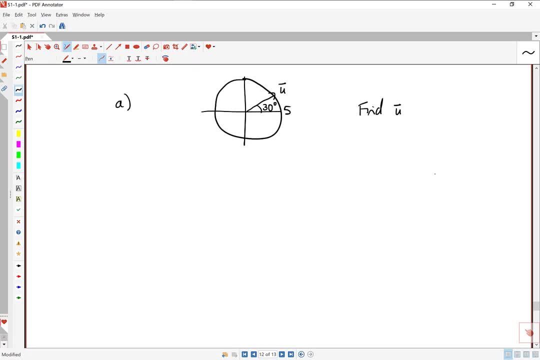 find vector u, so meaning just find the components of the vector. Okay, so let's think back to trig. We're going to draw our special thirty, sixty, ninety triangle, so that's thirty degrees there. hopefully you remember the side lengths of that triangle. That's one. 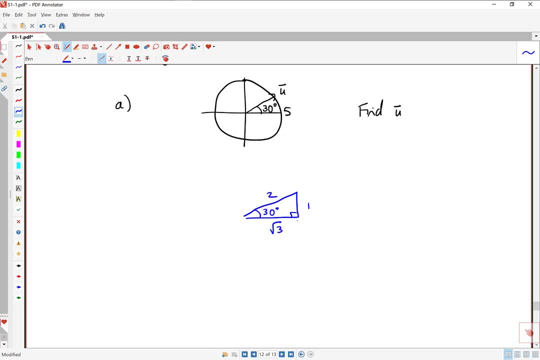 root three and two: Smallest side across from the smallest angle, longest side across from the biggest angle. and then what we're going to do is just scale this up, because the fact that this circle has radius five tells us that this vector here has length five. 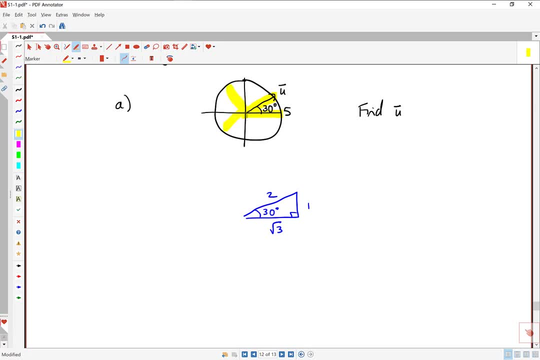 Any ray out from the origin to the circle is going to have length five. So what we want to do is just multiply this triangle by a constant to create a situation where the hypotenuse has length five. So if we multiply by five over two, 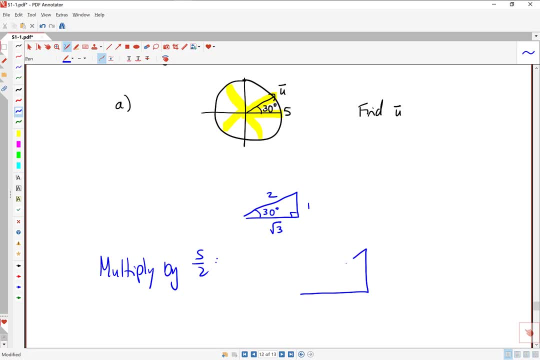 that will scale our triangle perfectly. So then we'll have five on the hypotenuse, five halves here, and this is going to be five root three over two. So this vector that's going up like this, that's our vector u, and we can now write down its components. 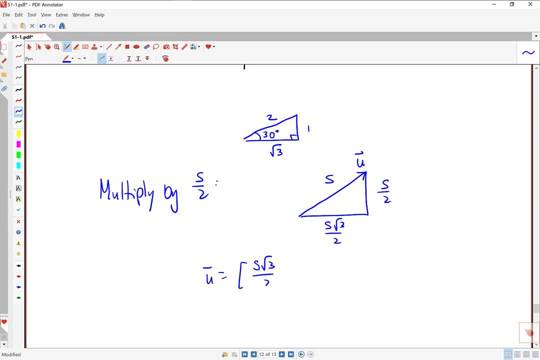 So horizontal component: five root, three over two, and vertical component: five halves. Again, let's say that we've got a circle centered at the origin and let's say, this time the radius is seven And this time we've got a vector that's going this way, making an 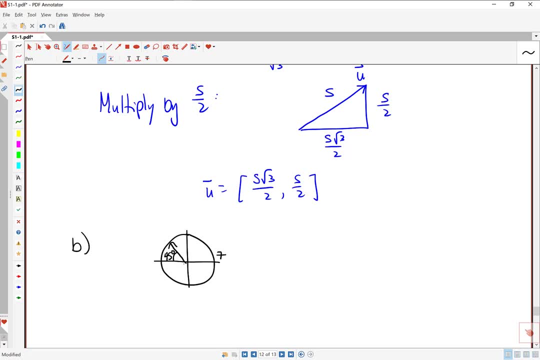 angle of forty five degrees with our negative x-axis. Let's call this v. So our goal is to find vector v. Okay, well, let's draw a triangle position like this: Forty five, forty five, ninety triangle. So from pre-calculus, our side. 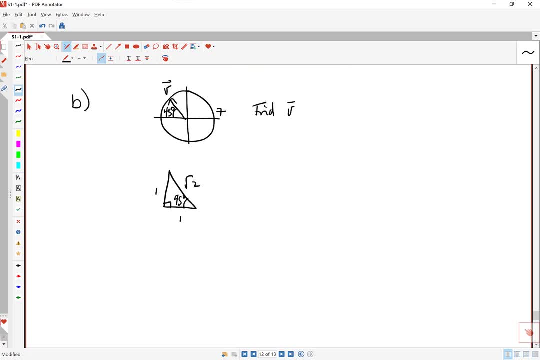 lengths would be one, one root, two and again. we want to do this idea of scaling it because if this circle has radius seven, then the length of v here is really seven. Any ray out from the origin to the circle is going to have length seven.